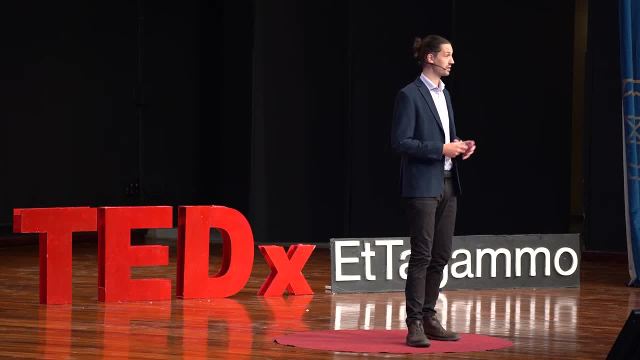 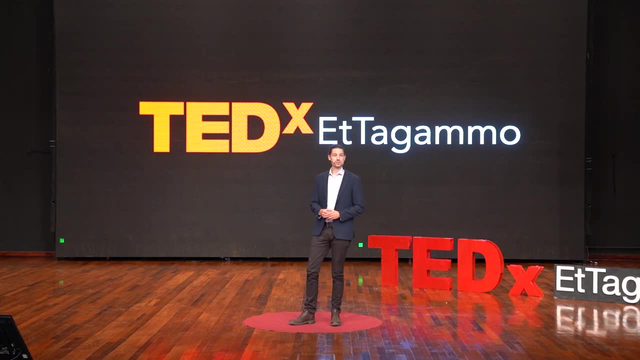 systems have a direct or indirect impact on us, whether we know it or not. The regenerative agriculture is mainly focusing on a holistic approach, focusing on soil health, the promotion of biodiversity, habitats and to create an ecological balance on the farm in order to 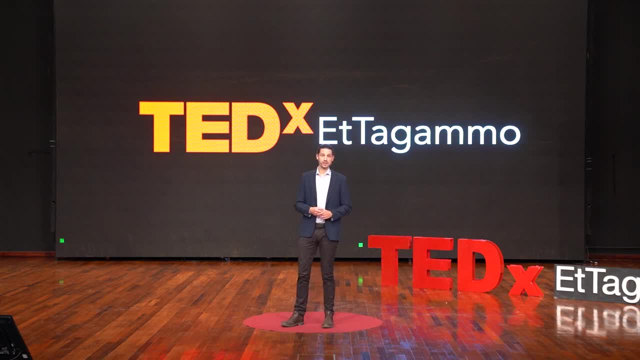 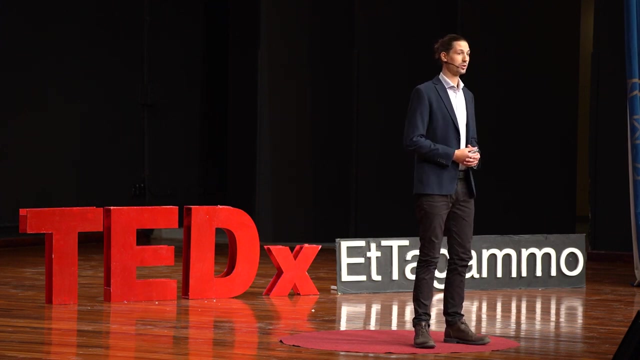 produce healthy products. The conventional system is mainly focusing on mass production and therefore also heavily relying on synthetic farm inputs, such as fertilizer, herbicides and pesticides, in order to artificially increase the yield. Luckily, my grandparents have one of the oldest organic farms in northern Germany, so I partly grew up on this farm and I was 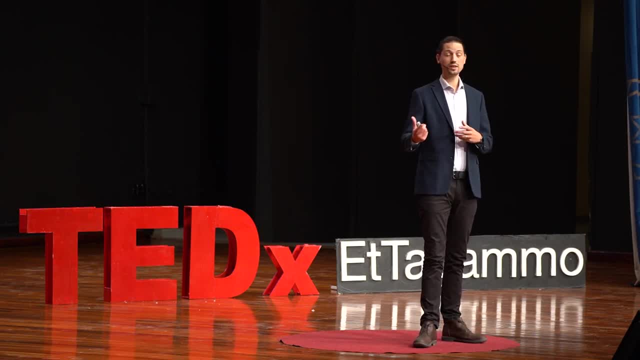 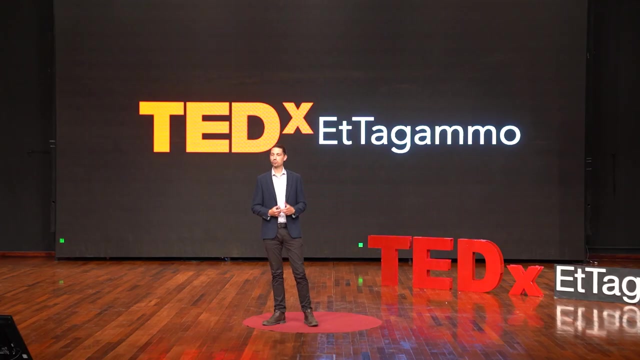 very connected. I think that the organic agriculture that I have developed since my childhood is in the nature and principles of organic agriculture as well. When I realized, when I learned that 98% of our global food system today is coming from conventional agriculture, I had the need and I wanted to explore how this conventional 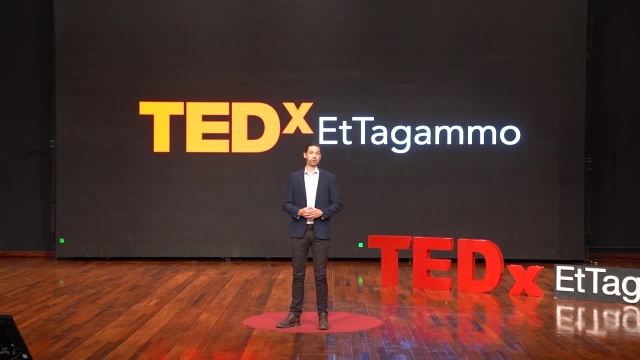 system looks like. So I decided to apply organic agriculture. So what can you tell us about the conventional system? working for a farm, a conventional industrialized farm in Australia, And working on this farm for several months has really changed my life fundamentally. 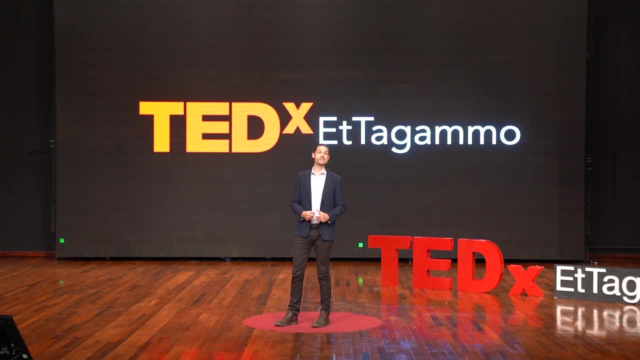 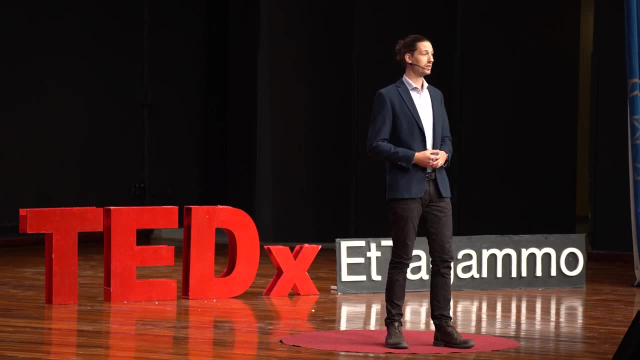 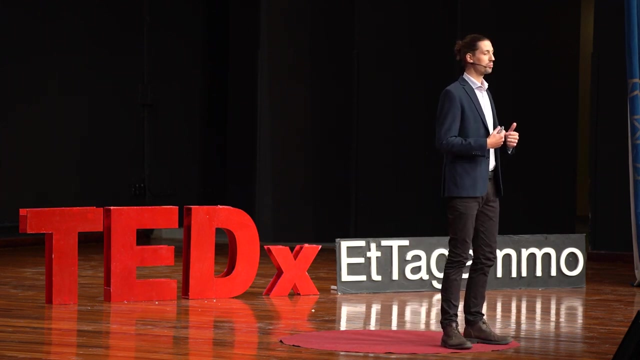 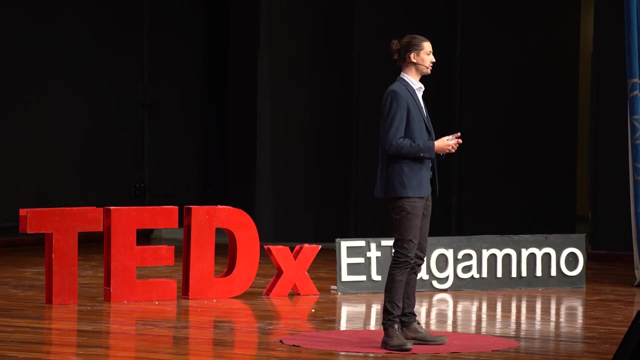 because I became part of an intensive disruption of natural ecosystems and, through my work, thousands of acres got burned down and thousands of acres got sprayed dead, And when I looked at this dead soil, I asked myself: how can we promote this? how can we promote a system that is largely responsible for today's 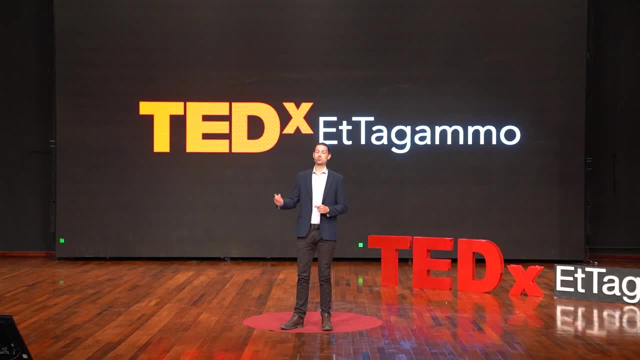 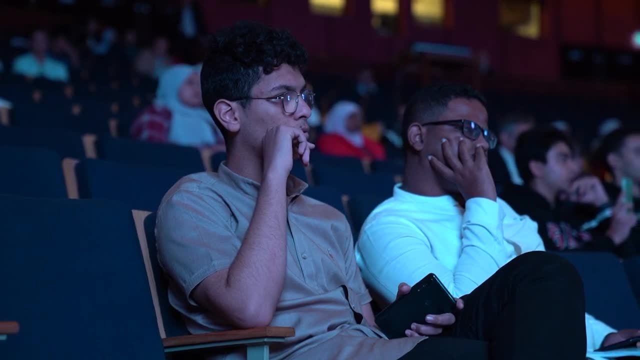 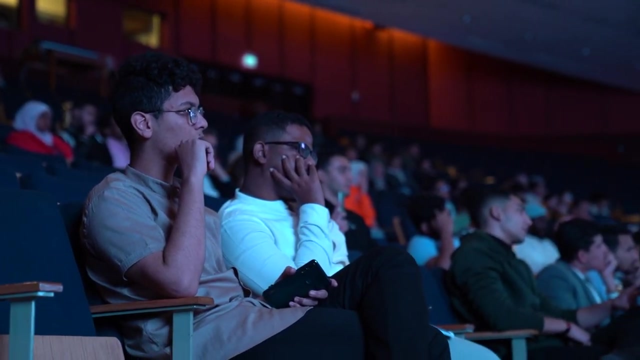 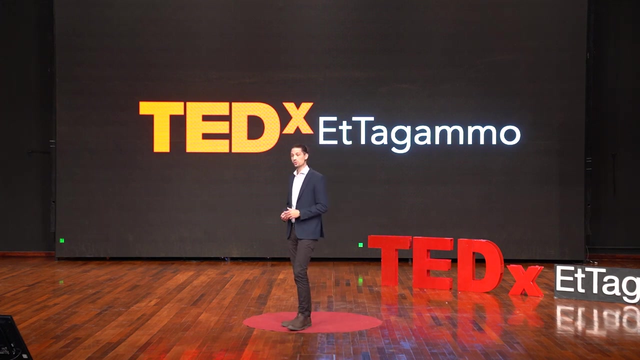 climate change and in the same time, is supposed to produce food for future generations and for our today's society. And when I found out that agriculture today is responsible for 18 percent of the global greenhouse gas emissions, some sources even say over 20 percent, and that agriculture also is 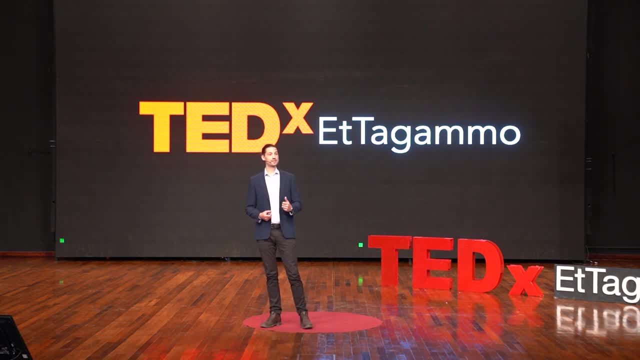 responsible for 88 percent of today's pollution of rivers and streams. I was quite shocked, And in addition to that, I learned that biodiversity loss that we are facing currently is also largely responsible and caused by the conventional agriculture, And here the biodiversity loss is mainly visible in the decline of wildlife, but also in the loss of food. 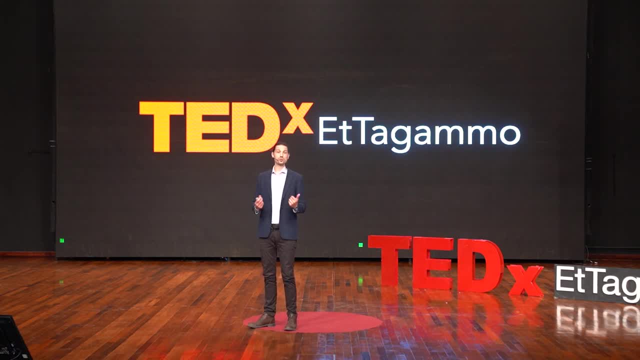 seeds, which in the end makes our systems less resilient to pests and diseases and other climate change events. And when we see that over 40 percent of today's insects are in decline and threatened, we might think- or we tend to think- that biodiversity loss does not really affect us. right, We live here in the 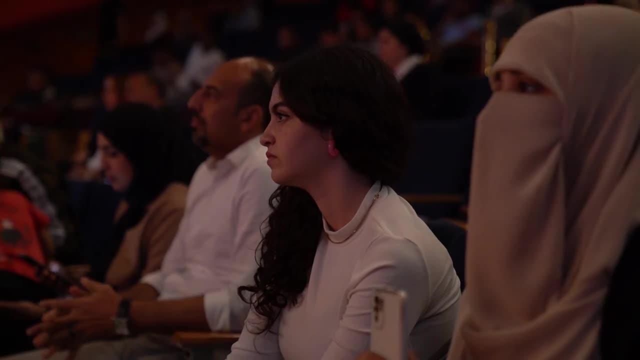 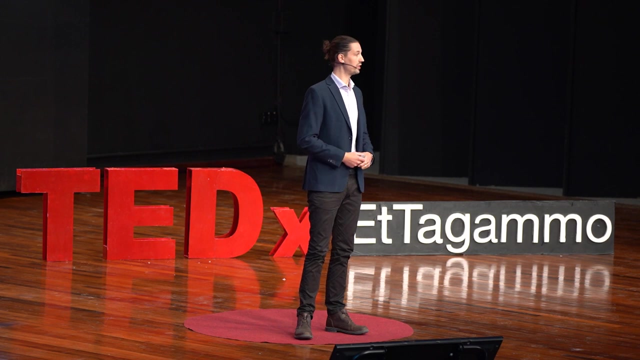 cities in Cairo. how should this affect us? Maybe, except on having less insects on our windshield while driving on the highway compared to 30 years ago. But if we continue like that, we might not be behind the steering wheel after next 30 years, because 35 percent of our global food supply today is heavily 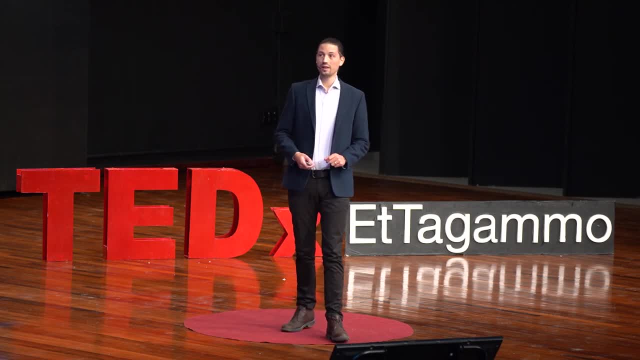 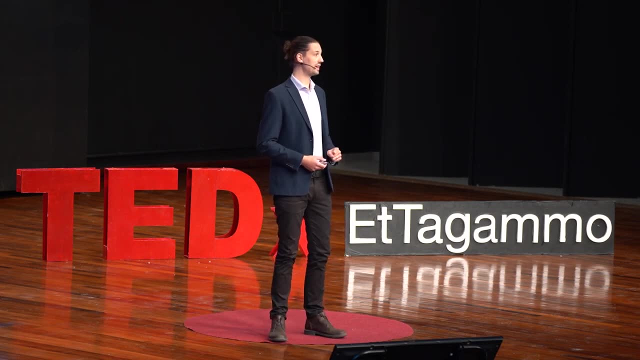 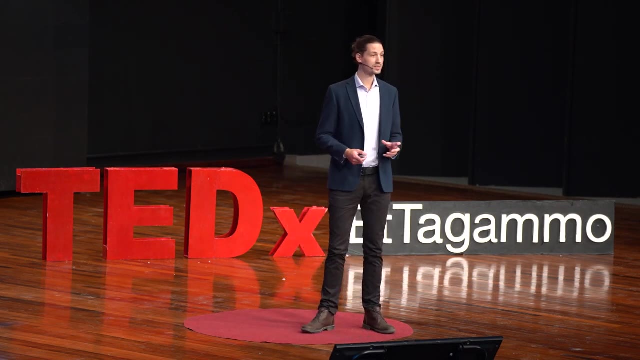 dependent on those insects. Now, if we compare the conventional agricultural system with the regenerative, we quickly realize that the regenerative agriculture provides a huge ecosystem service to society which is at the moment not being taken into account and not being valued, And through 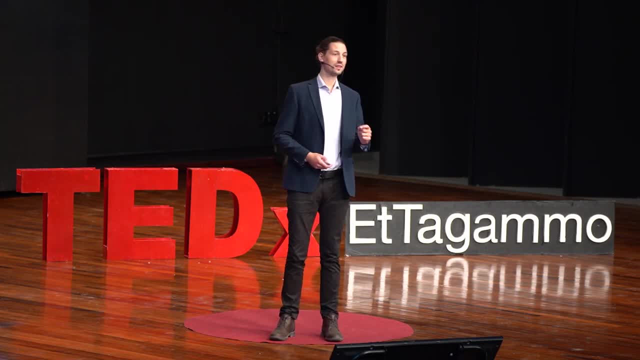 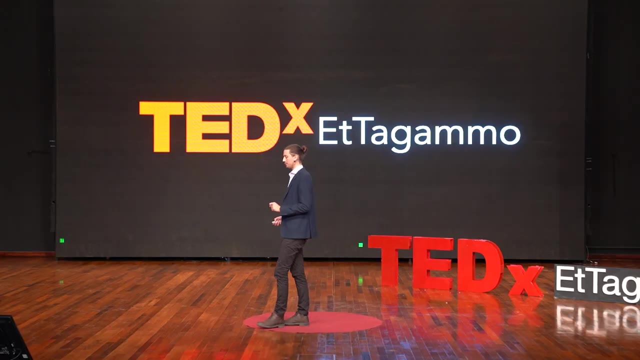 my work in this field, I realized that the regenerative system can only be scaled if we are able to provide a financial benefit to the farmers and to the communities on the ground that do the work And, besides supporting Egyptian farmers, of producing healthy food for the society we have started to measure. 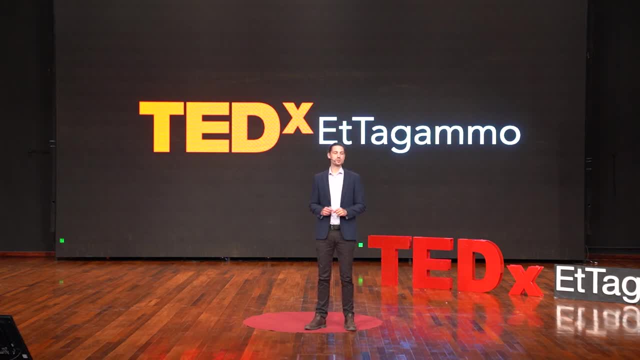 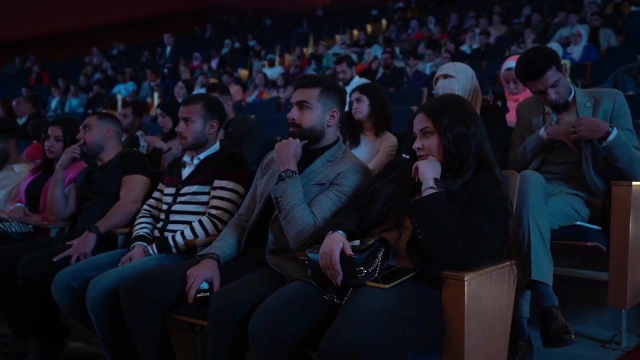 and incentivize farmers for the ecosystem services, And this is mainly happening through that. we measure how much carbon, how much CO2, can be stored in the trees that are surrounding regenerative farms. It also is about how much carbon, how much CO2, we can sequester in the soil through crop rotation, cover crops or 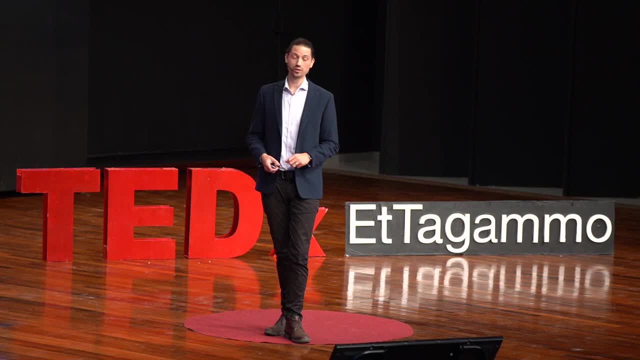 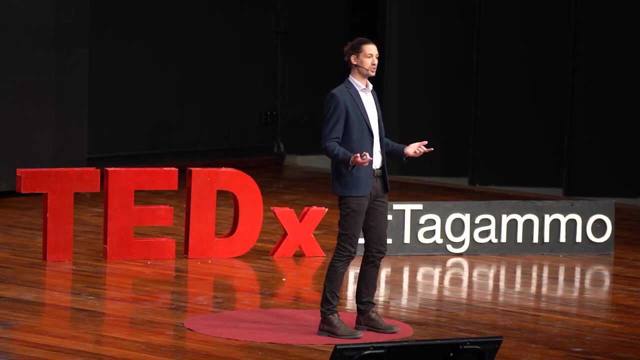 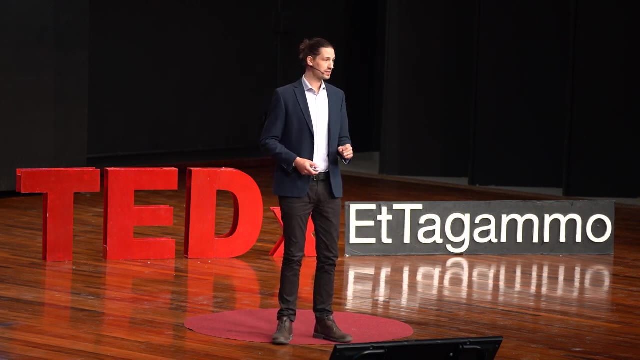 other regenerative practices. We also take into account the compost that is produced on the farm, because by producing compost we can avoid a lot of methane emissions And we can take this into the equation. And if we are installing renewable energies on the farms, of course this enables us as well to decrease the carbon. 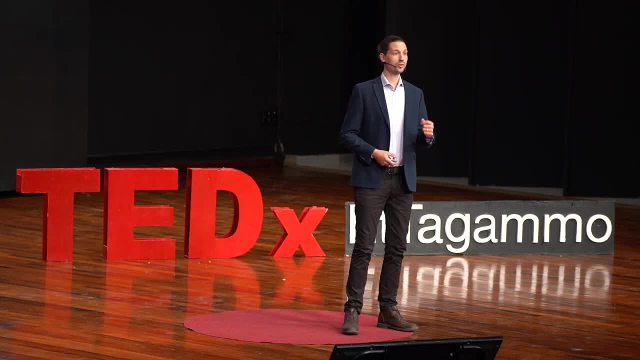 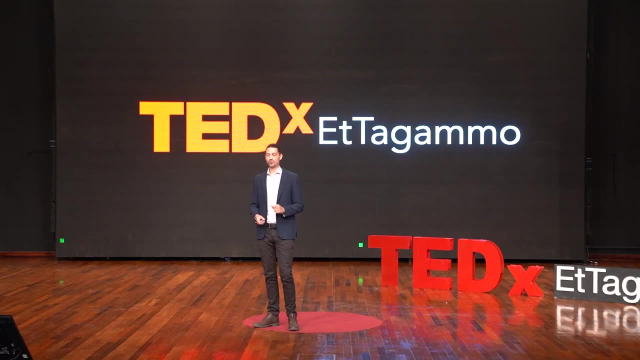 emission because we are not dependent anymore on the irrigation pumps, the diesel pumps that we need for irrigation. So along the way, I realized that agriculture can either be a powerful carbon sink or one of the biggest emitters. And if we now look to the Egyptian context, we see that the conventional agriculture here in Egypt is emitting CO2 to the atmosphere- two to five tons of CO2 per acre per year, whereas the regenerative system has the potential to sequester and avoid up to 11 tons of CO2 per acre per year. 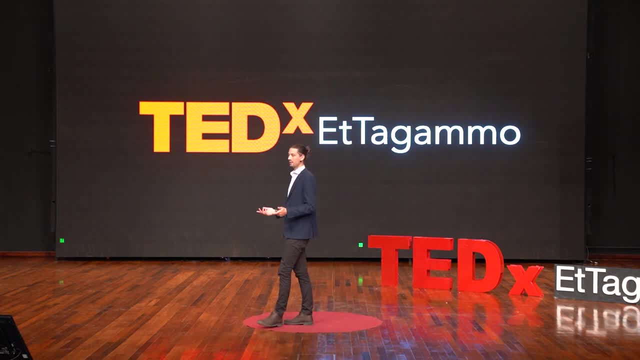 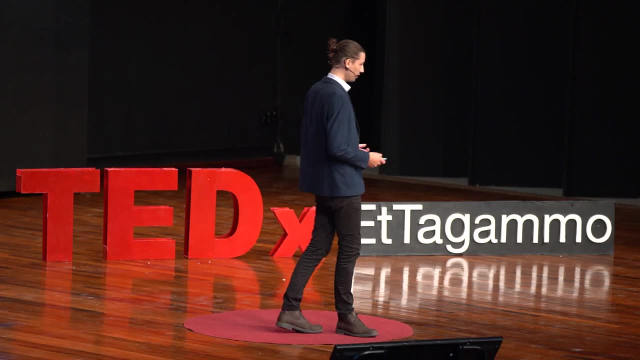 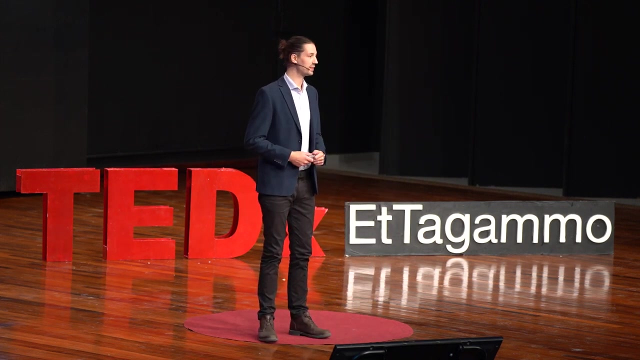 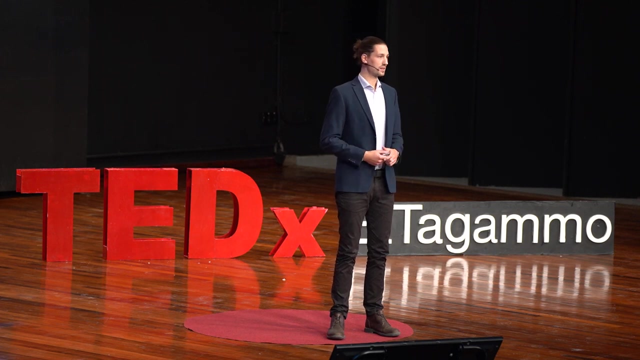 And if we see those numbers, we can clearly say that agriculture has a great potential of mitigating climate change. right, And actually, in the end, the farmers on the ground should be appreciated for the services that they are doing. And now a lot of farmers and a lot of people already around the 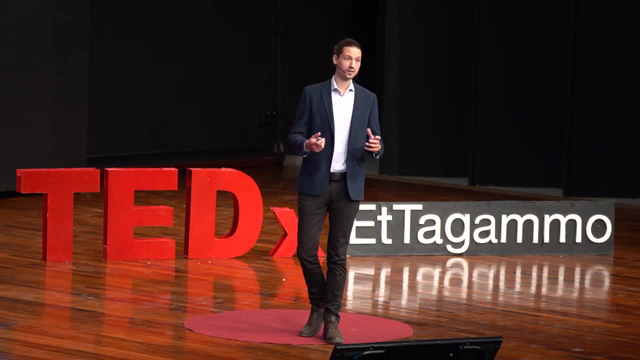 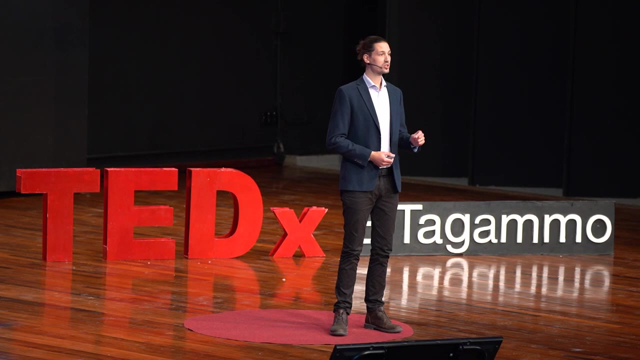 world are applying regenerative agriculture And and organic agriculture, but they are not being incentivized for their services. But today we are using new methodologies by IPCC and UNFCCC to really measure the performance that our farmers are providing on the ground, And 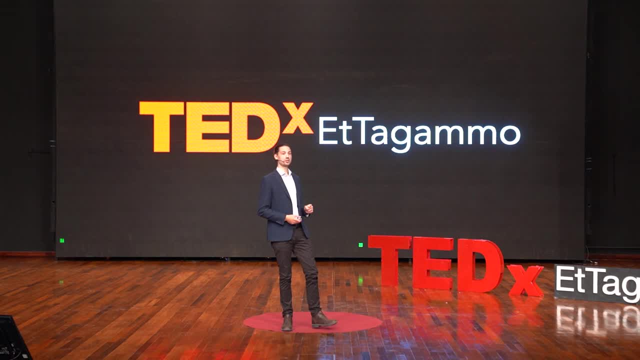 currently we are working with around 3000 farmers in Egypt and scaling up to 40,000 farmers within the next two years. But now imagine if all Egyptian farmers would apply regenerative agriculture. we would have a potential of sequestering and avoiding up to 100 million tons of. CO2, which is around one-third of Egypt's total emissions today, Isn't that great, And actually the value of those 100 million tons is around 3.5 billion euros, which is today 100 billion. The value of those 100 million tons is around 3.5 billion euros, which is today 100 billion.